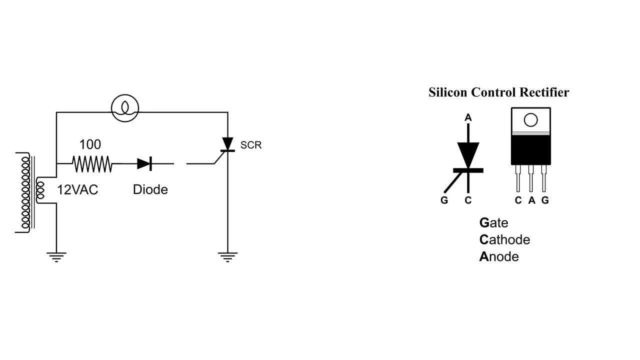 And the other side of the bulb to one side of the 12-volt AC. Now, when the AC is in this configuration, when we have positive and negative in this configuration from the AC supply and the gate is connected to the diode, 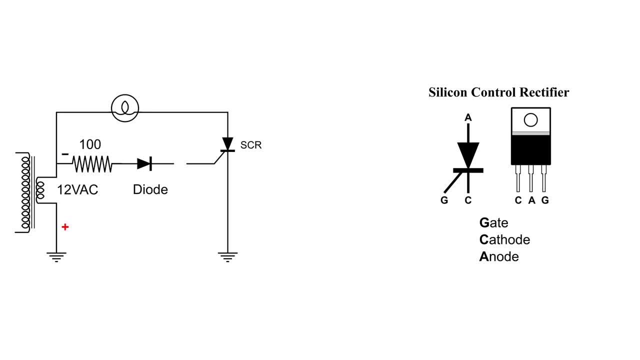 it will fire the SCR. But if the AC is in this configuration- negative on the top and positive on the ground- even with the gate connected to the diode, the bulb will remain dark, But of course not for long, because this is 64 hours cycle. 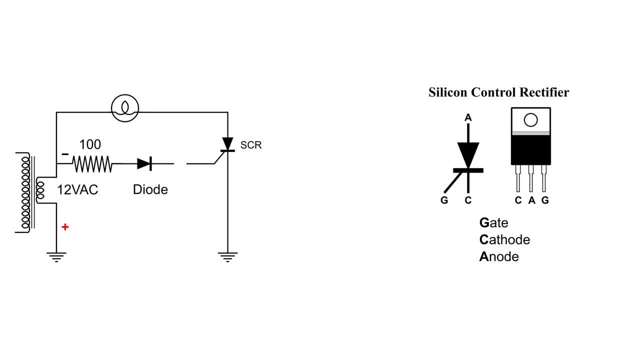 so it's all thanks to drums and students that can help us to make things even better. to get the other half of that circuit, I added a little more to this diagram: another 100 ohm resistor, another diode and another SCR. but notice the configuration it is in the circuit in the opposite direction of the SCR on the 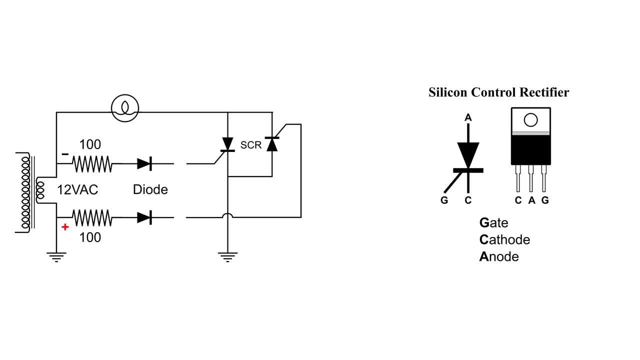 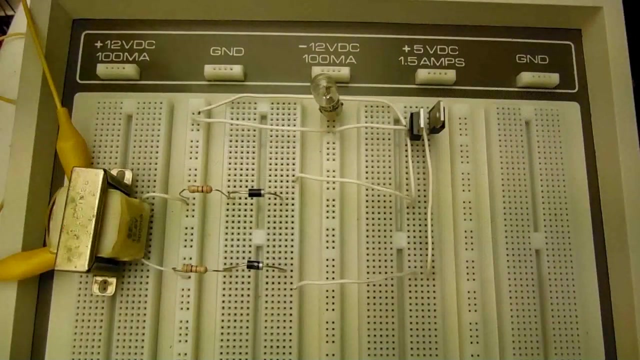 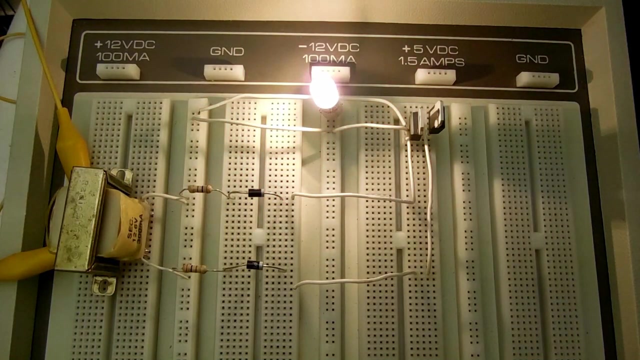 left in this configuration, having the positive on the ground and having the diode connected to the gate. the second are the right. most SCR will fire lighting the bulb and here's a video demonstrating that. I'm going to connect the top lead- a diode- to the gate of the left SCR and the 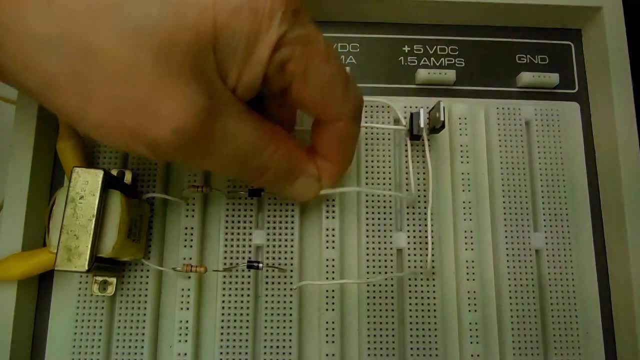 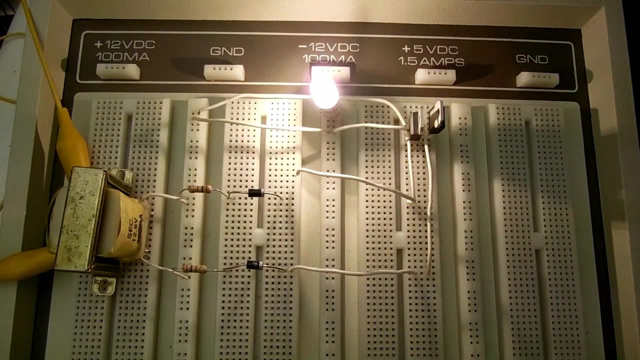 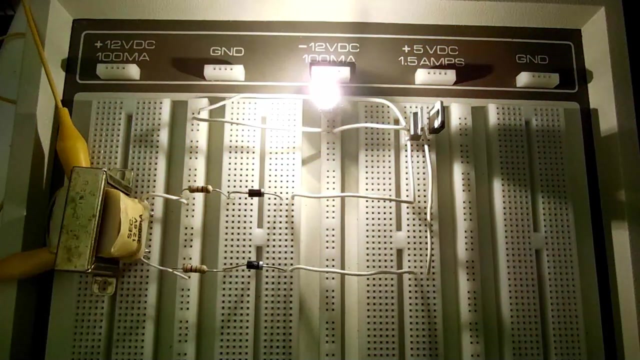 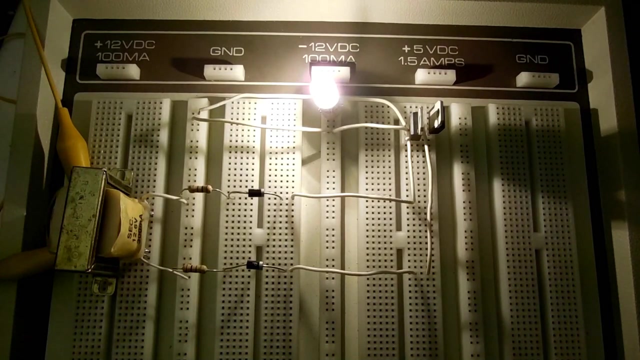 bulb lights. disconnect that and connect the bottom lead, a diode to the gate of the right SCR and the bulb lights again. I'm also now going to connect the top lead and you can see the bulb got much brighter. the camera is turning down the light here, but the bulb with both leads.